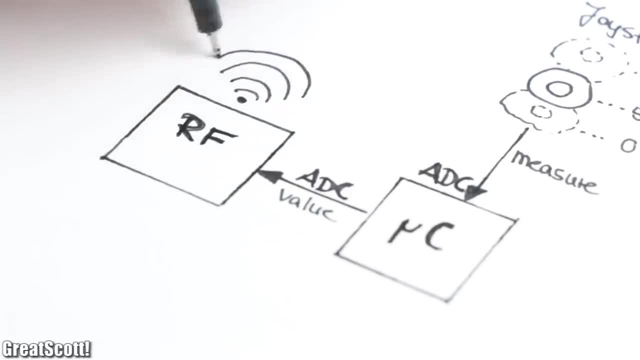 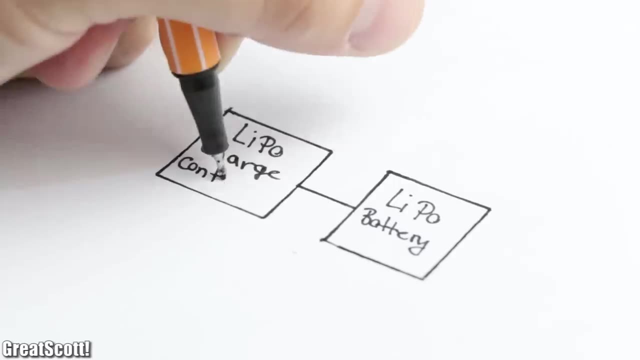 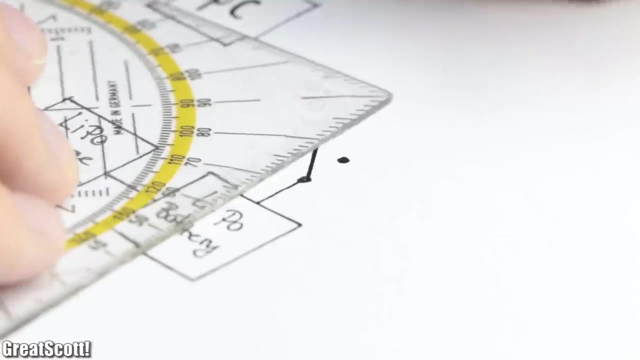 joystick and then sends the values through the RF band to a receiver. Also, I wanted to power the circuit through a LiPo battery, which means I needed a LiPo charge controller IC, a micro USB port to deliver the power for charging and a power. 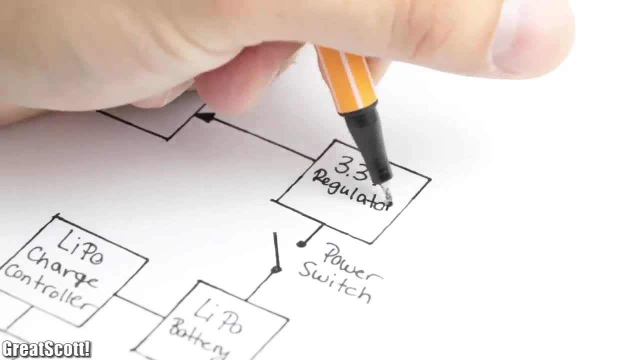 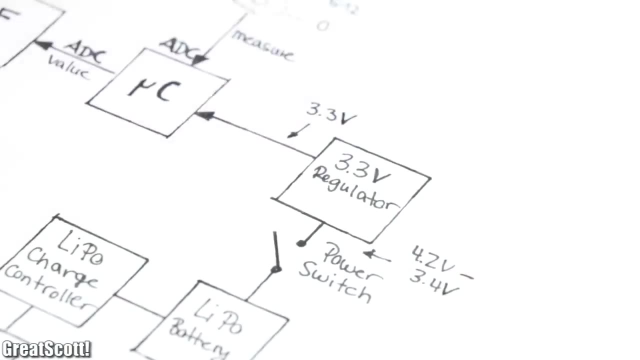 switch to connect the battery voltage to a 3.3V regulator which converts the undervoltage, the unregulated battery voltage, into a suitable voltage for the microcontroller. Last but not least, I wanted to monitor the battery voltage through a voltage divider with. 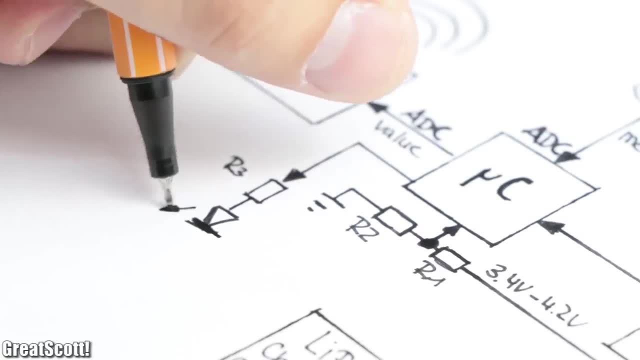 the microcontroller so that, when the battery voltage gets close to 3.4V, the RF functionality shuts down and a yellow LED lights up. And with the function of the circuit planned out, it was time for step 2, which involves: 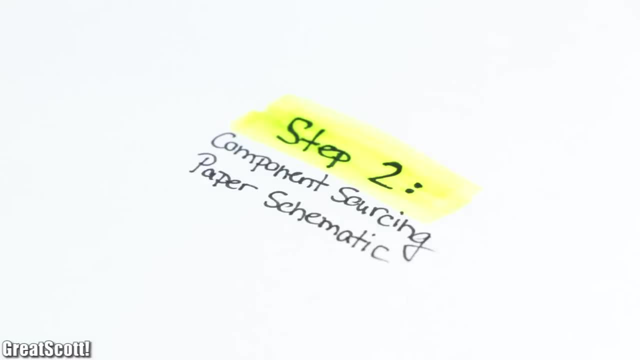 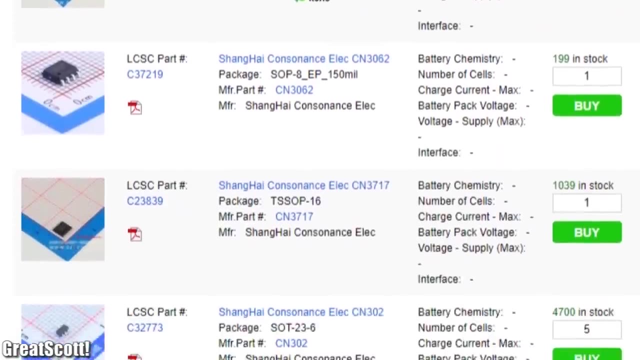 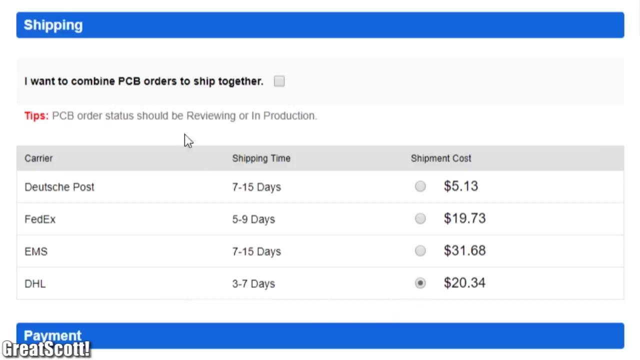 searching for suitable components and creating the circuit For component sourcing. I like to use LCSC because their selection is not only big, but also because we will be ordering the PCBs through JLCPCB later on and we can combine that with the LCSC order and thus save shipping costs. 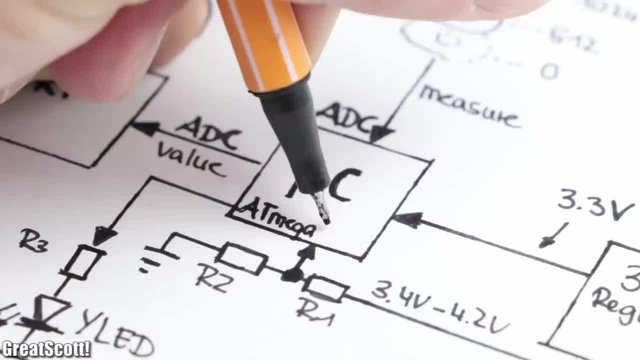 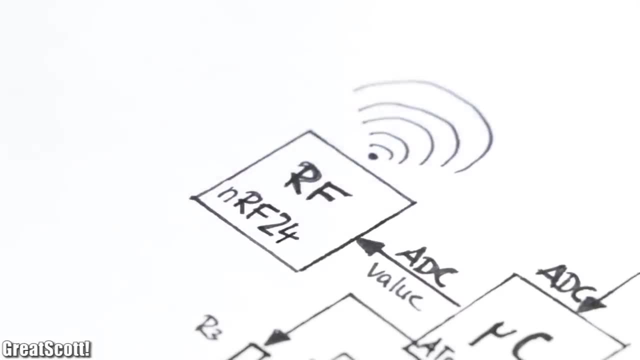 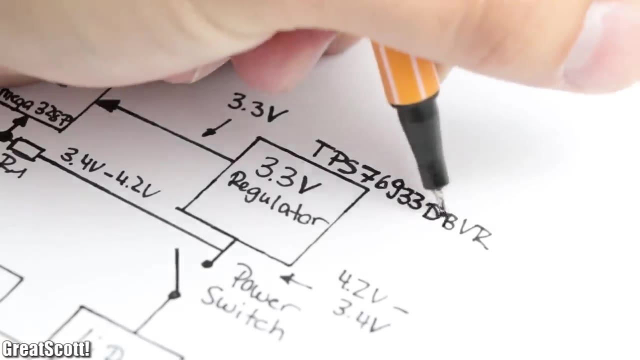 But anyway, once I decided on the main ICs, which were the ATmega328 as a microcontroller and NRF24 as a microcontroller, I decided on the ATmega328 as a microcontroller and NRF24 as a microcontroller. I decided on the ATmega328 as the RF transmitter, a TP4056 as the charge controller and a TPS76933. 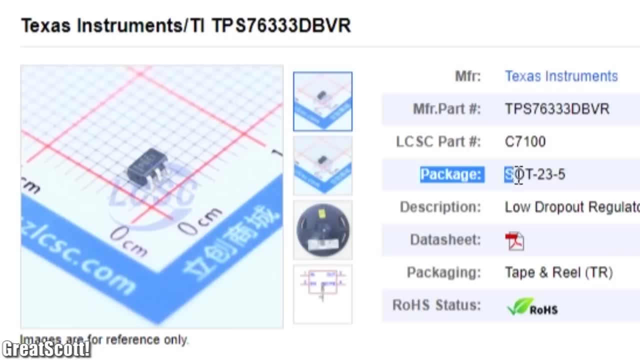 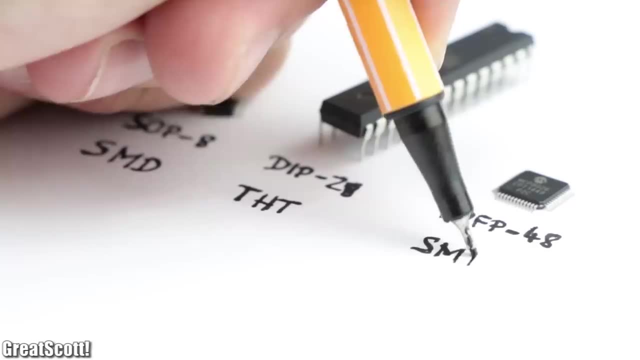 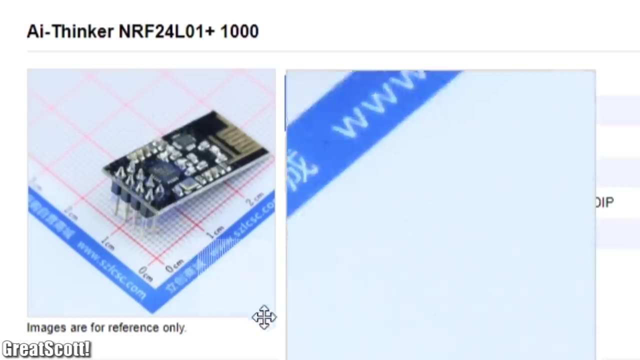 DBBR as the voltage regulator. It was time to think about the packages. The package basically describes how the IC will physically look like and determines whether it is a THT or SMD component, For example, while the NRF24 is only available as a breakout board and THT, it is also a 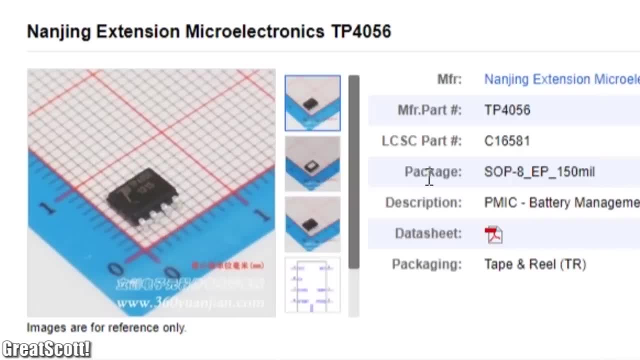 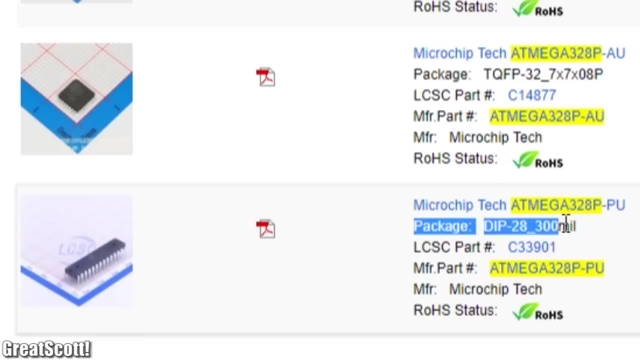 TPS76933 DBBR and the TP4056 is only available as an SMD version. we do have the choice between THT and SMD for the microcontroller, But since I wanted the circuits to be as small as possible, I went with the SMD version. 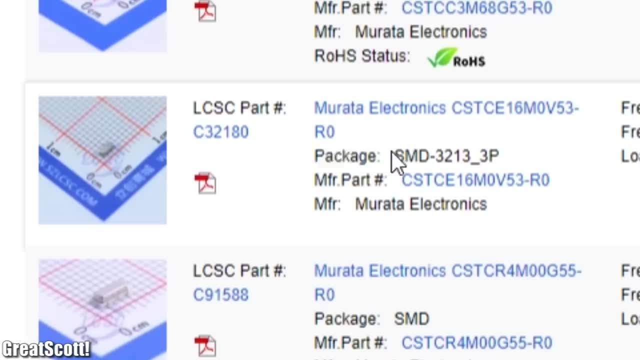 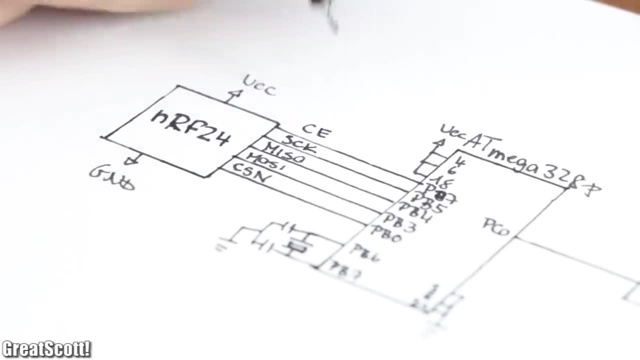 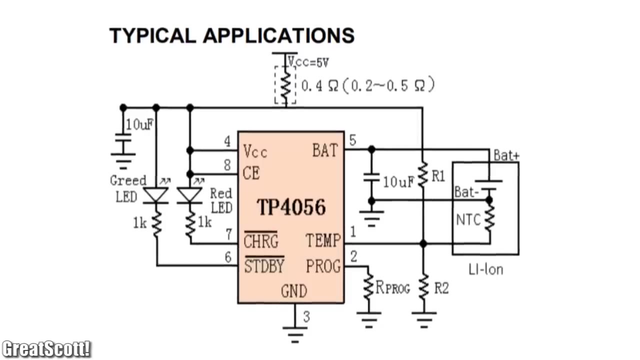 which I also set as the standard for the remaining complementary components. Next, I planned out on a piece of paper how to connect the main ICs to one another and also what passive components are necessary to make them all work. To find that out, I had a closer look at all the datasheets of the ICs and their recommended. 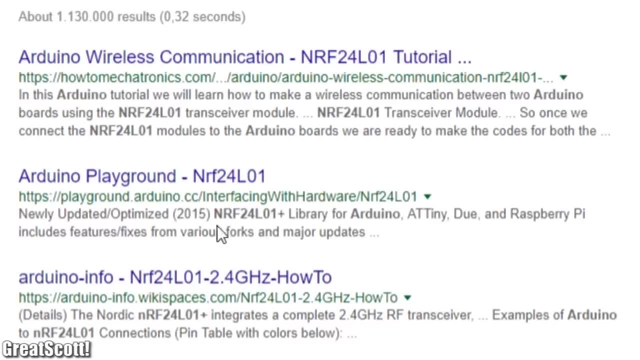 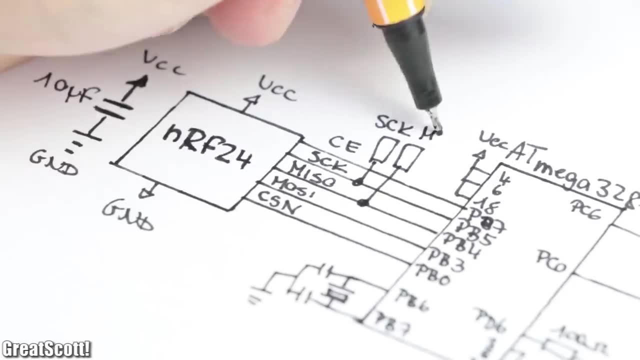 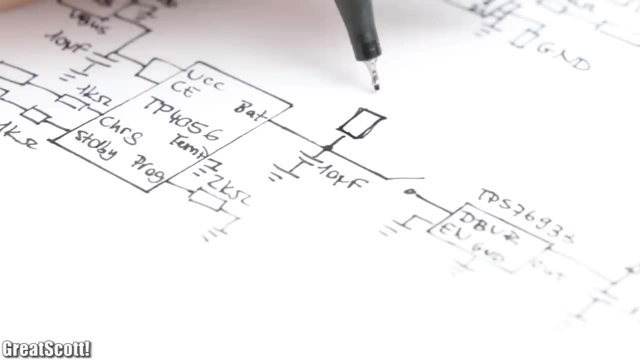 example circuits, and if everything fails, you can always google your question, which should give you a suitable answer. in 99% of the cases. The last thing to do for the paper circuits was to add breakout points so that I could later program the microcontroller and also hook up the battery and LED's. 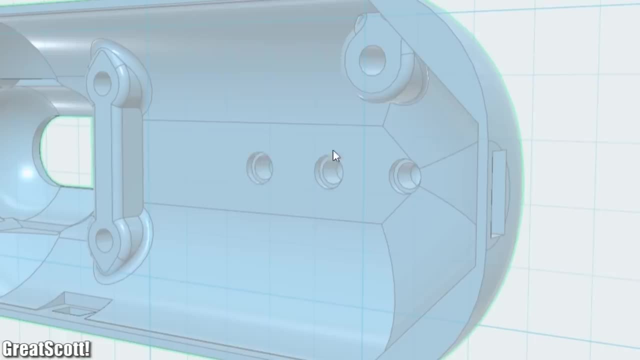 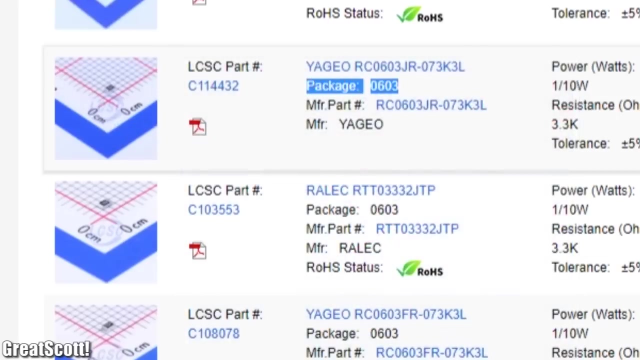 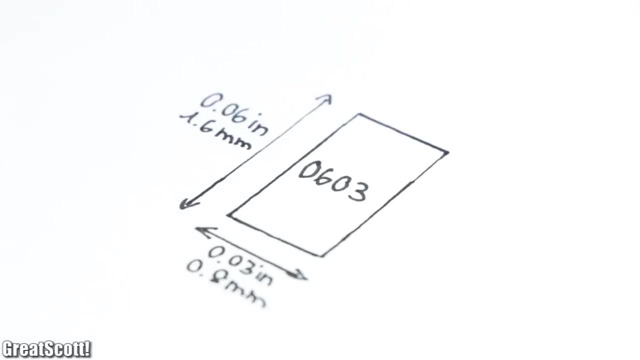 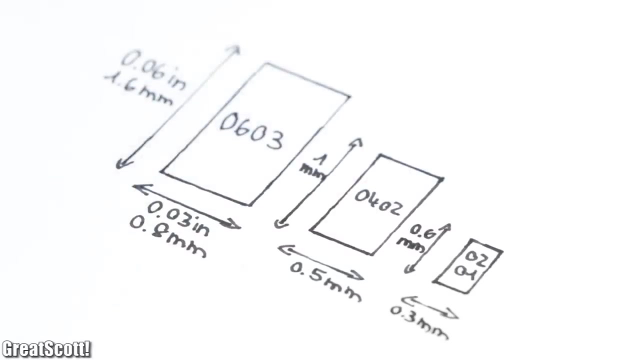 Now for the passive component selection. I mainly went with 0603 as the package size, which stands for 0.06 x 0.03 inches or 1.6 x 0.8 mm. There also exists a 0402 and a 0201 package, but I think 0603 is neither too big or too. small and can still be sold separately. So I decided to add 0603 as the package size. Now for the passive component selection. I mainly went with 0603 as the package size, which stands for 0.06 x 0.03 inches or 1.6 x 0.8 mm. 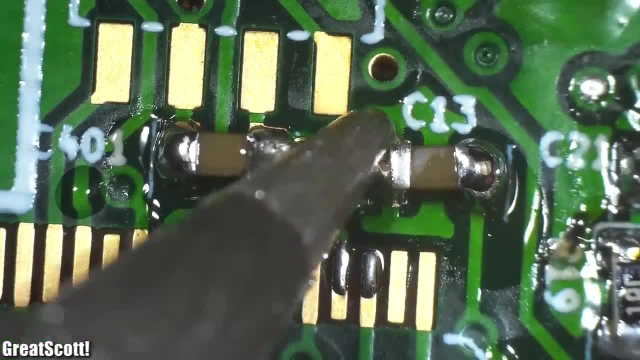 So I decided to add 0603 as the package size, but I also think 0603 is neither too big or too small and can still be sold separately, Since I currently use the preserve and render mode, the. This will be the complete basic думаю, and also on the server server. 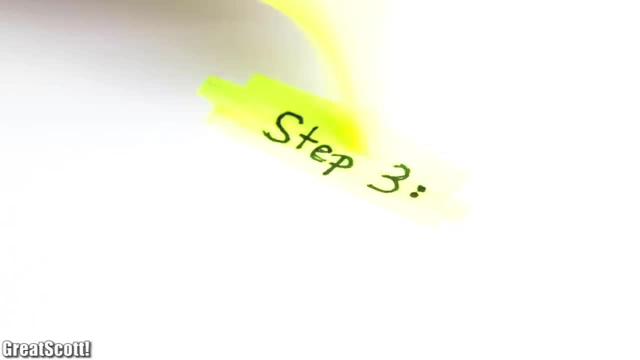 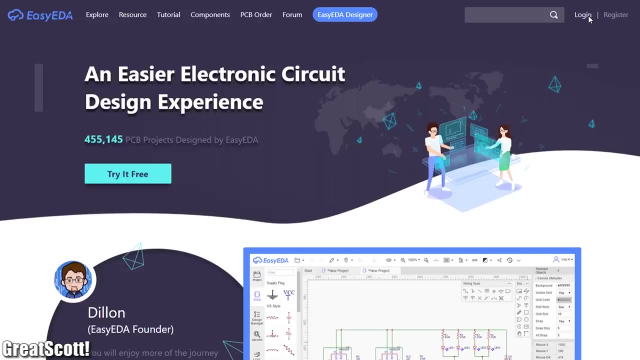 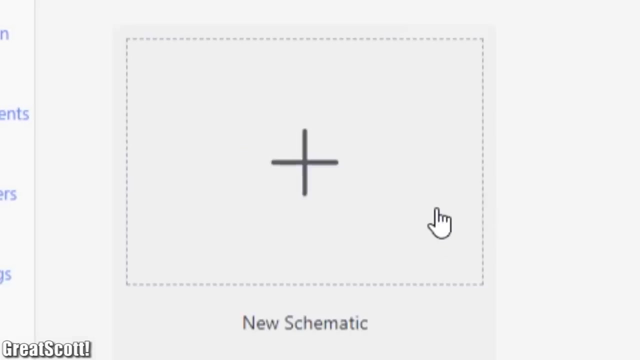 And with the component selection and paper schematic being completed, it was time for step 3. Creating a proper schematic. For that I used the EasyEDA FreeOnline Circuit Creator. After logging in, I created a new project and there a new schematic. Then I simply used their online library, which also includes pretty much all LCSC components. 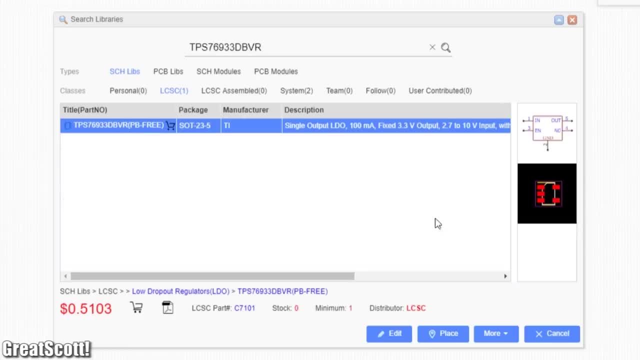 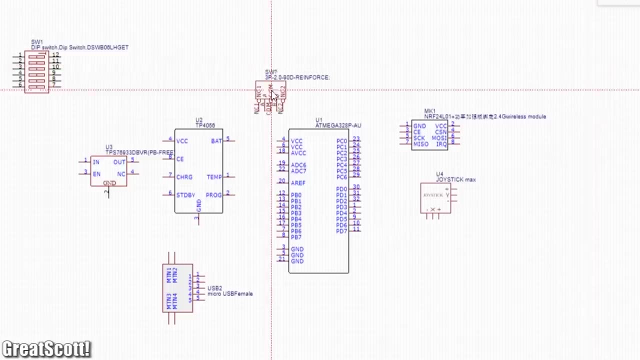 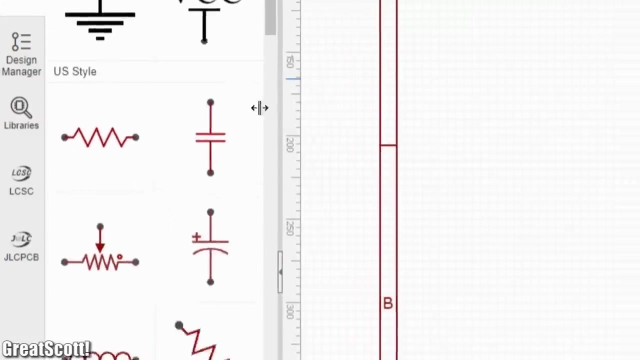 to search for my utilisation components and firstly imported them into the workspace. but make sure that you choose components with the right package and correct footprint, otherwise the PCB design will later not work out. Once all the main actors of the circuits were imported, I then used the left aligned resistors with the right package. 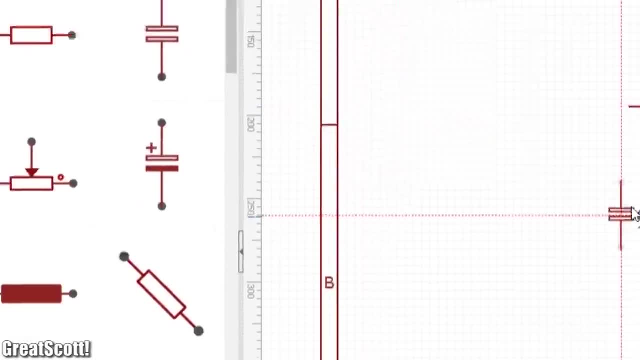 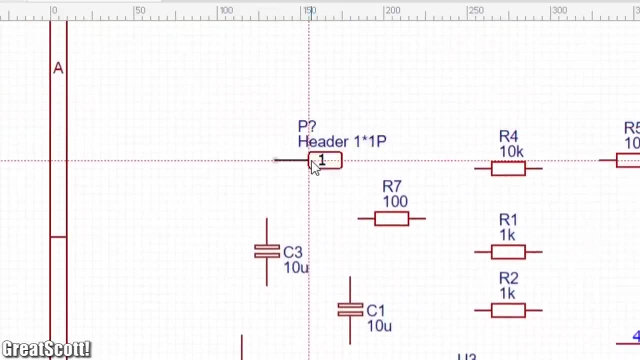 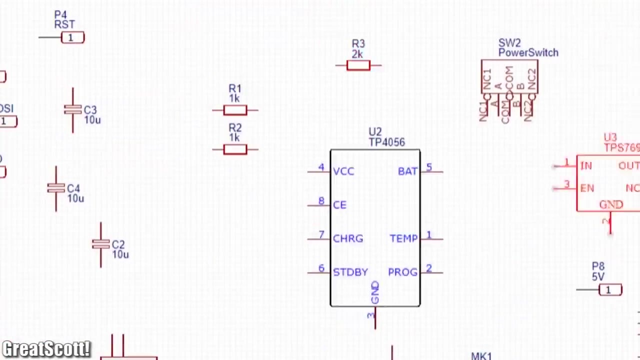 and capacitors with the right package as the complementary passive components, and, of course, we should not forget to add male header connectors for the breakout points. Now that we got all of our required components in the editor, we can arrange them to logical blocks, which in my case is the power parts and the 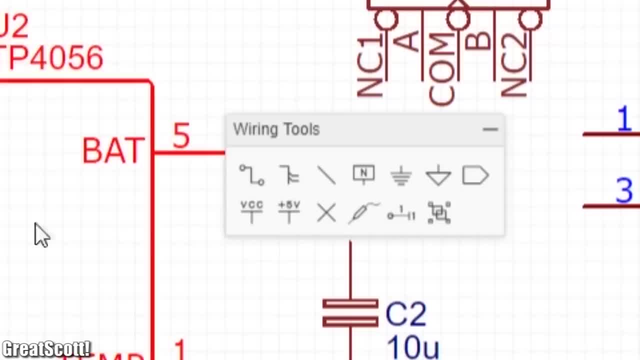 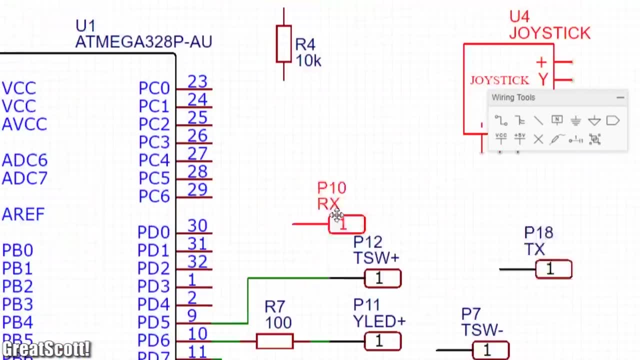 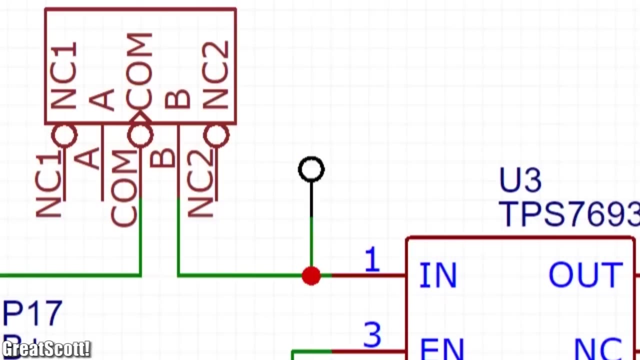 microcontroller parts. Once that was done, I utilized the wire function of the software to connect all the components to one another, according to how I planned it out on paper. Last but not least, I then added the ground VCC and battery voltage supply flags to the schematic, which not 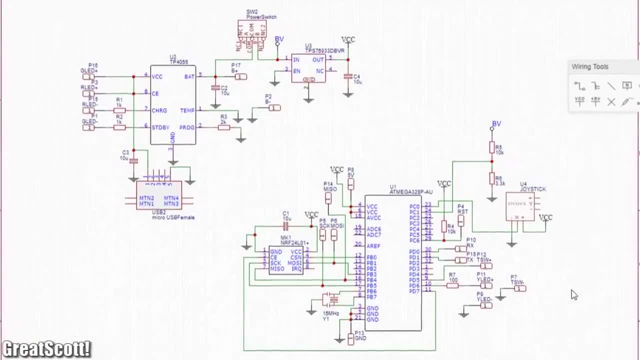 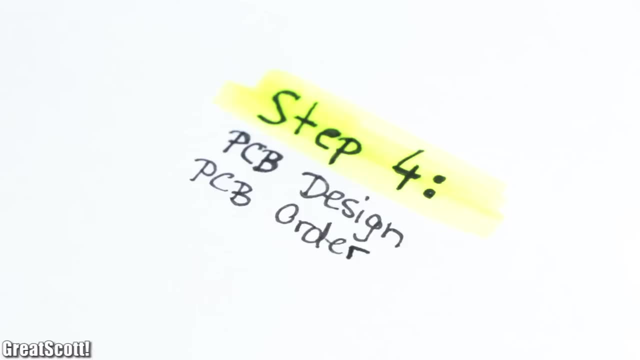 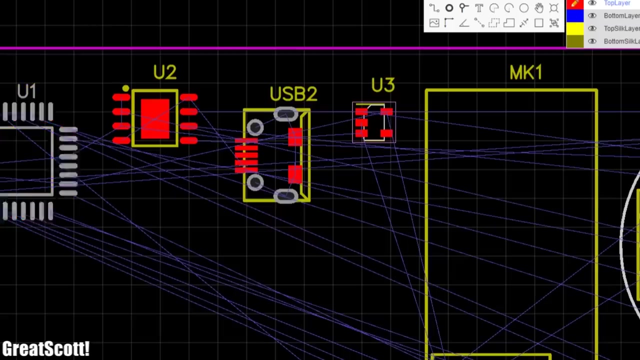 only completes it but also ends the third step of this tutorial. That means it is time for the last step, Step 4, which is PCB design and ordering. For that we firstly have to click the convert to PCB button, which automatically throws all the component footprints into the PCB editor. shows how to connect them. 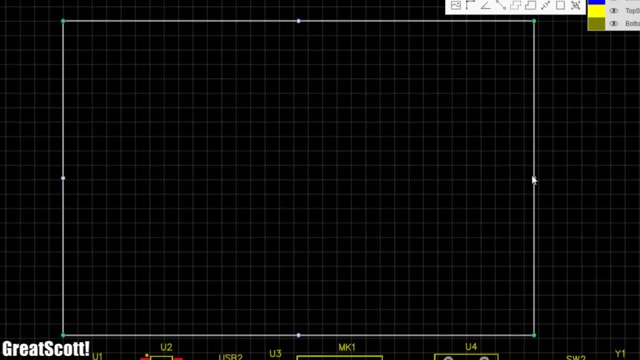 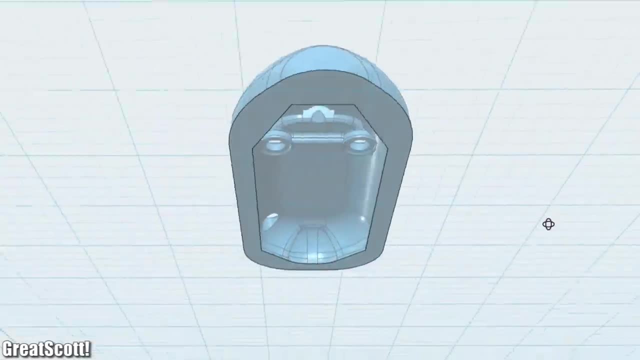 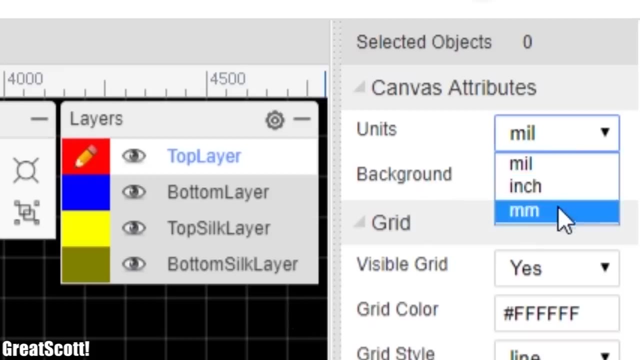 through the blue lines and creates the circuit. The first thing I did, though, was removing the outline, because, as I mentioned earlier, I needed a specific PCB size for the enclosure. To do that, I changed the measuring system to millimeters, selected the board outline layer and used the track tool in combination. 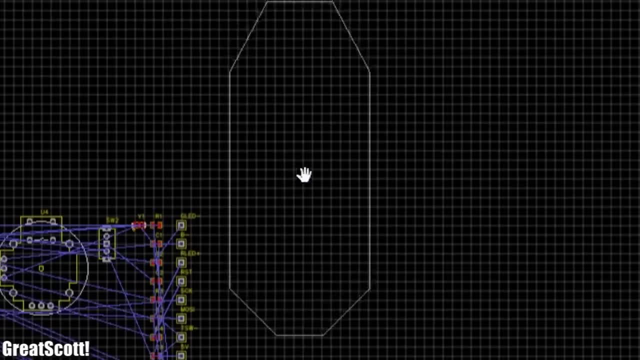 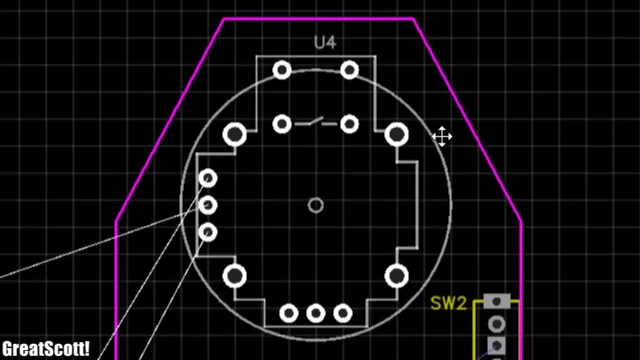 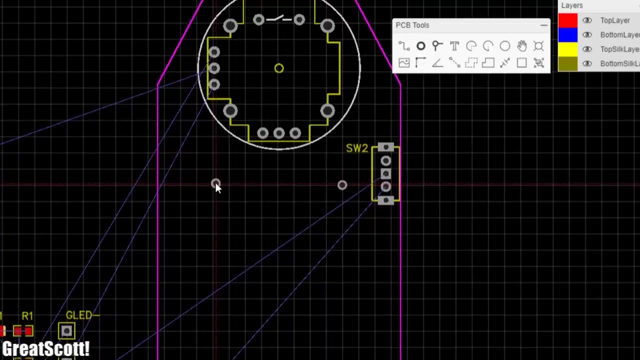 with the given coordinates in the down right corner to create the correct size for the PCB. Then I moved the micro USB port, the memory and power switch and the joystick to the required position, according to the enclosure's cutouts, To later mount the PCB. I also added 3 pads. 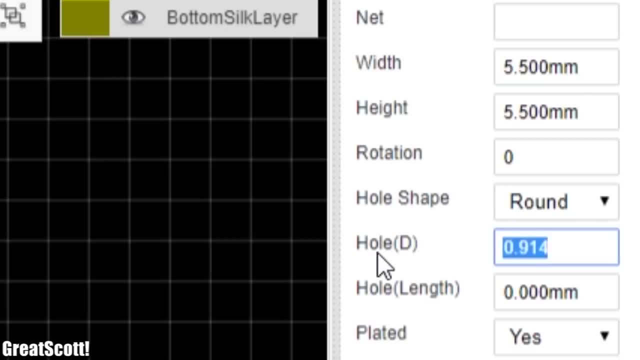 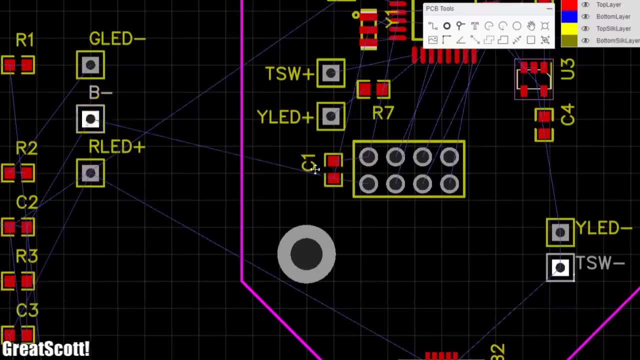 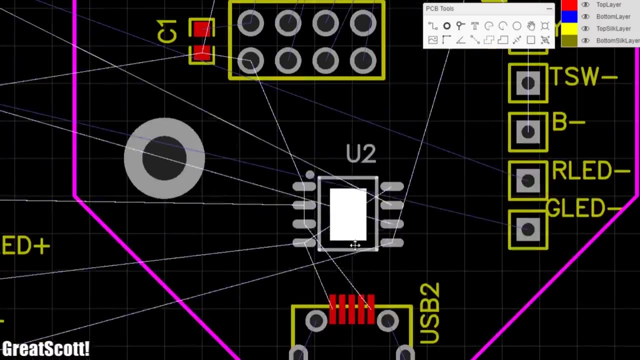 whose size I enlarged so that M3 screws would fit through them, And, with that being done, I placed the rest of the components onto the PCB. Of course you want to separate the power part and microcontroller part a bit and also make sure that the pins slash components that need to get. 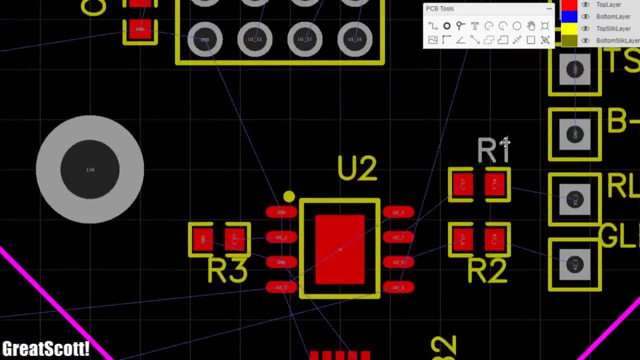 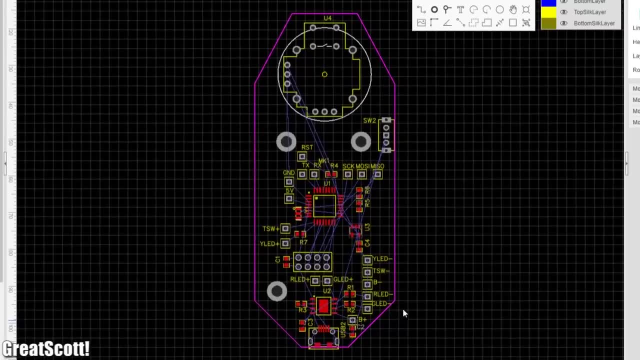 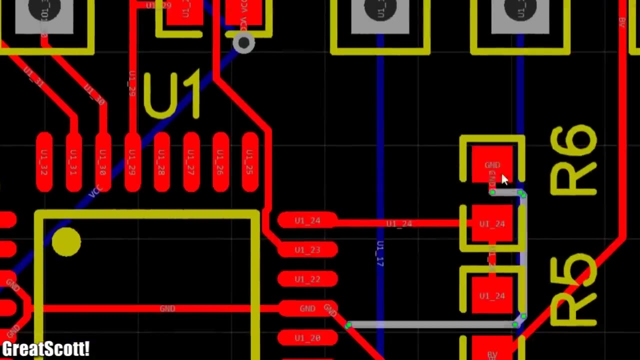 connected to one another are physically close to one another, so that the copper trace length can be as short as possible. As soon as you think your layout looks logical, we could use the given autorouter to do the wiring for us, but, as you might already have guessed, that is often not the best solution. 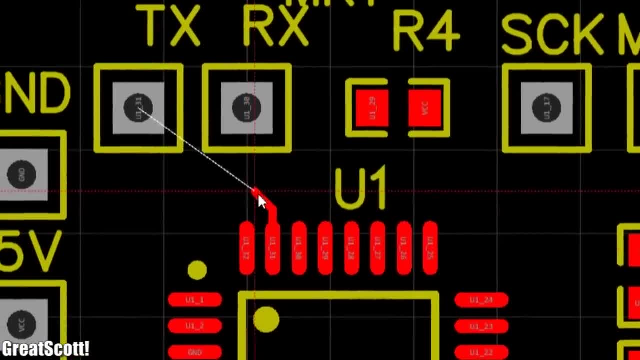 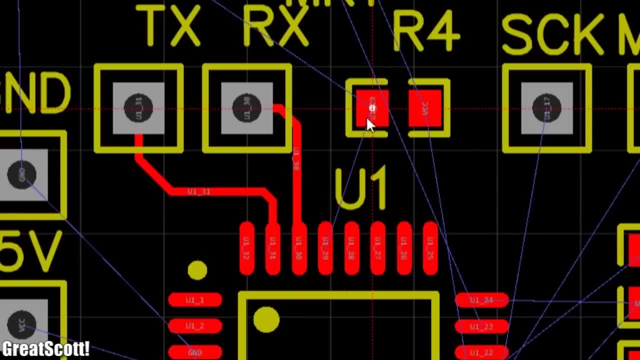 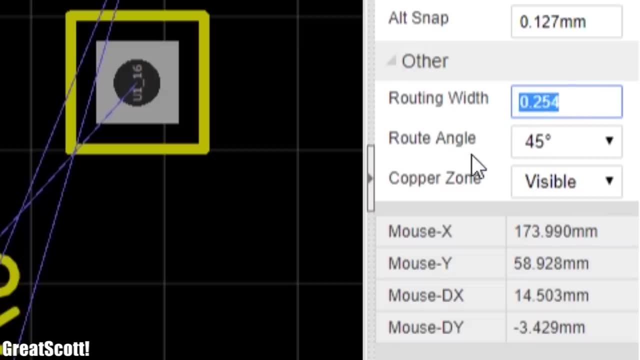 So let's do it manually, by selecting the top layer and using the track tool to simply connect all the components to one another. But before doing so, we have to talk about the width of the traces, which is usually set to 0.254mm. 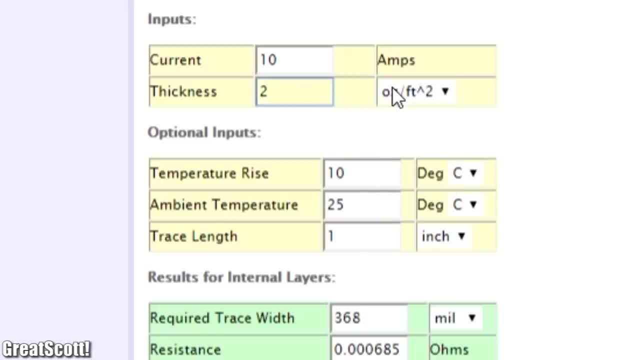 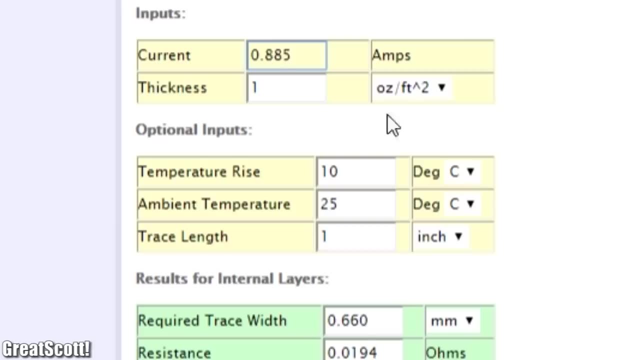 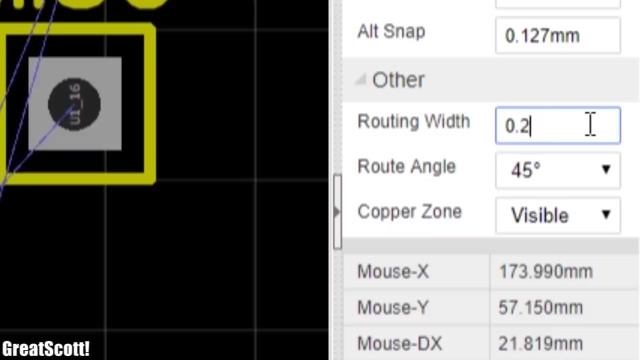 If we use an online trace width calculator and set the ounce value to 1, which is the standard value for JLC PCBs, then the trace could handle around 0.885A of current on outer layers, which is enough, but I always like to work with a width of 0.3mm. 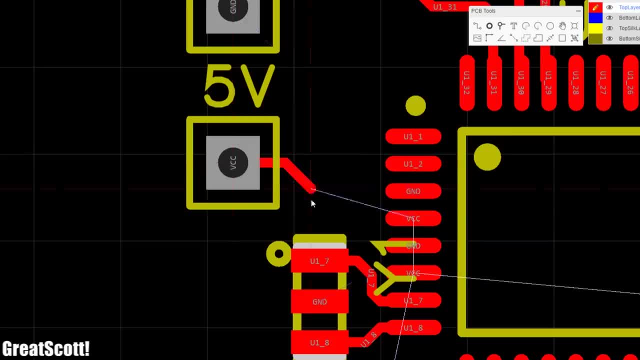 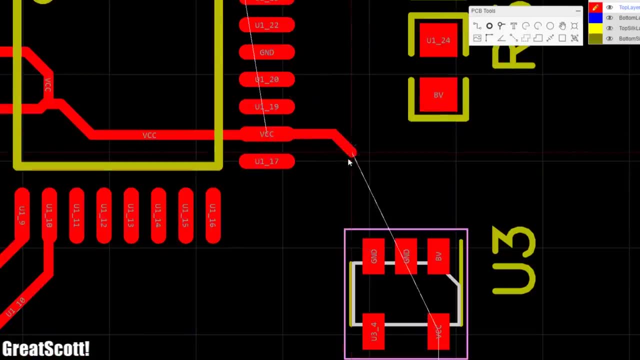 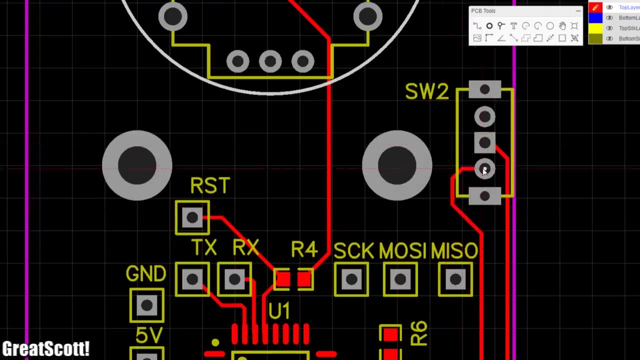 Since that gives me a maximum of 1A, And with that out of the way, I created all possible connections on the top layer, while making sure to not use 90 degree bends, since that is bad practice and everyone in the comment section will hate you. 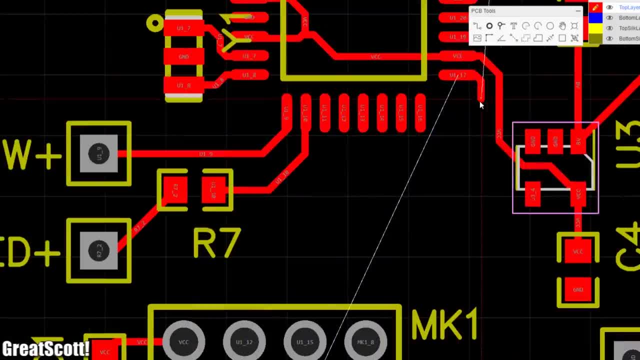 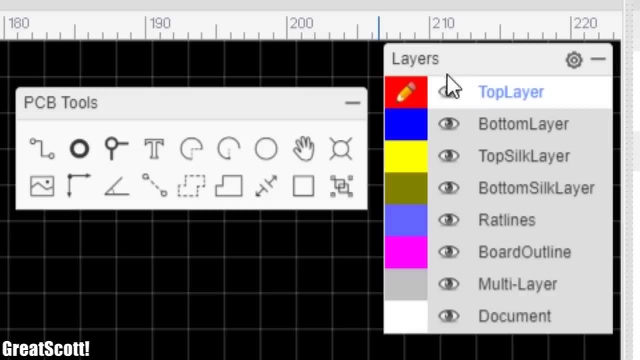 The only problem with this top layer wiring was that after a short while I was running out of space and not all necessary connections were made yet. But don't worry, Since we can switch to the bottom layer and do the rest wiring there, which would be very 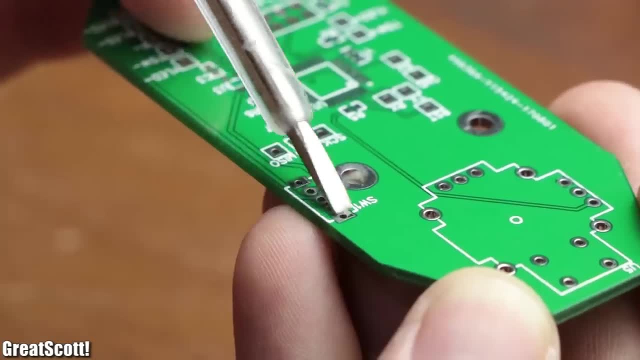 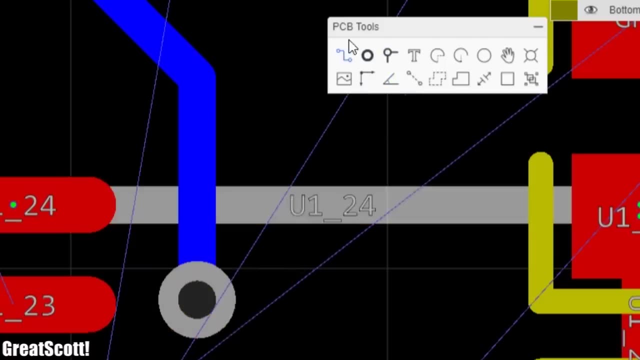 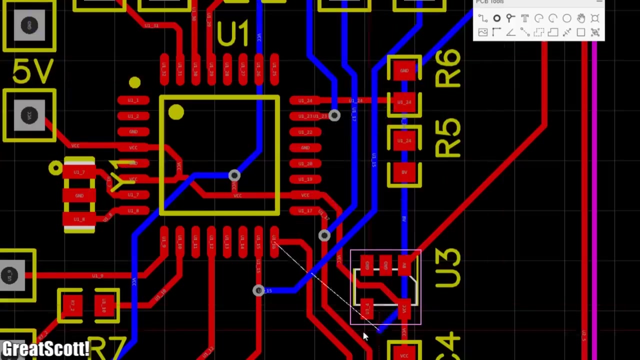 simple to do for THT components, since their solder pads penetrate through all layers, But for SMD components we have to create a so called VR. It is basically a small tunnel that connects the top and bottom layer, and just like that we can finish the wiring even for SMD components on the bottom layer. 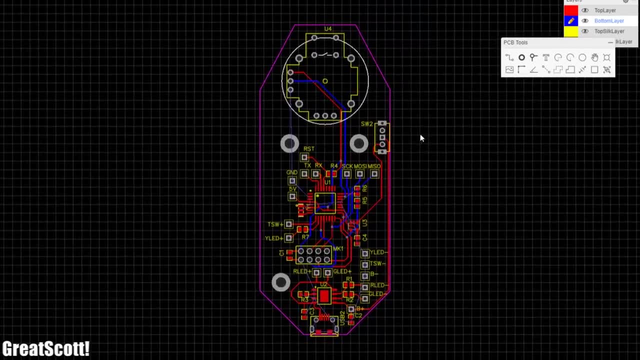 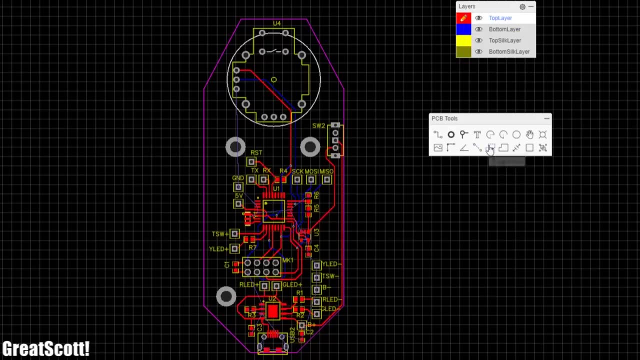 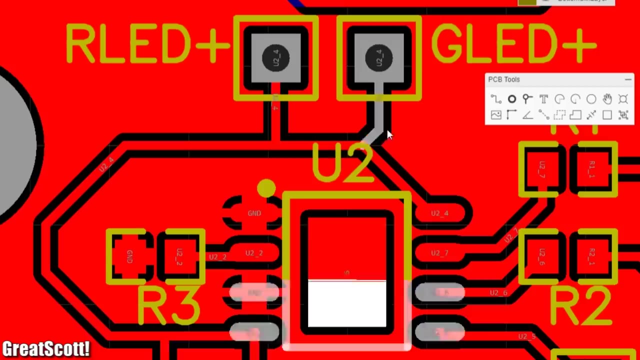 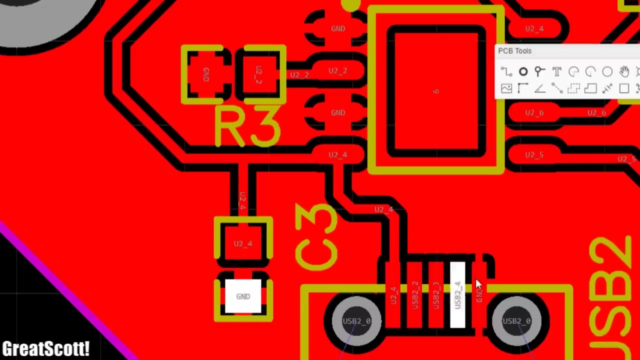 Now here is my finished PCB design. Well, for those, we can simply select the top layer and use the copper region tool to encircle the whole PCB And just like that, the traces got isolated and the rest of the top layer space is used as a solid copper ground layer. 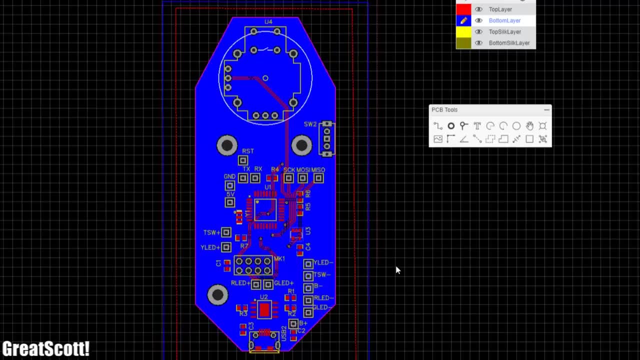 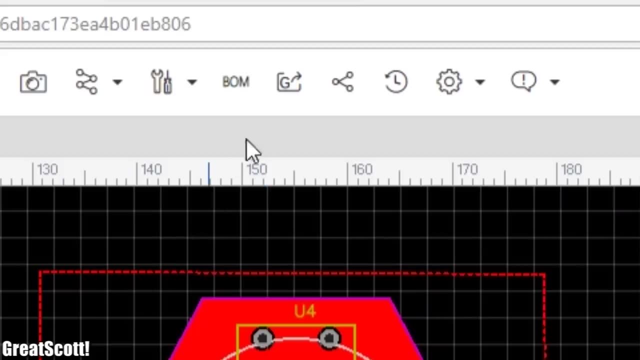 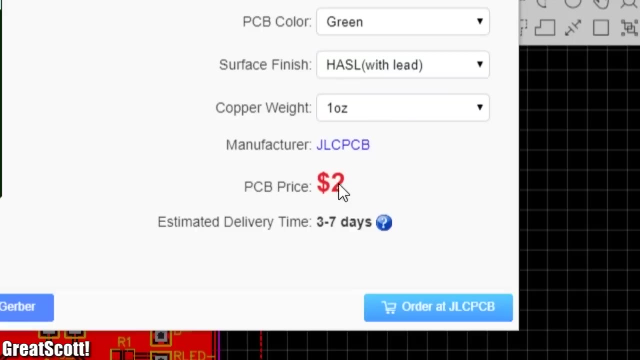 Of course, if you want to, you could also repeat this process for the bottom layer. At this point, the PCB design is basically finished, Which means we can click generate Gerber files in order to download them, or we can directly order our finished product from JLCPCB, which I did.